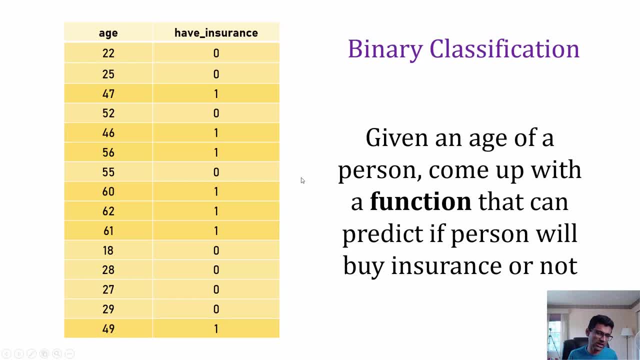 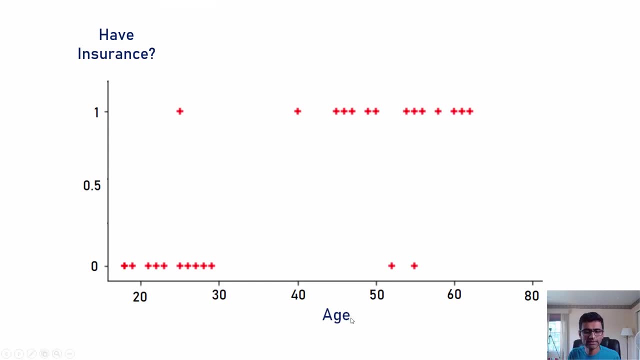 an algorithm that can be used for classification problem. so let's go over some theory. i am going to plot this particular data set on a scatter chart like this. it's a simple chart, my friend: x-axis, you have age, y-axis, you have zero, and one zero means person doesn't have insurance. 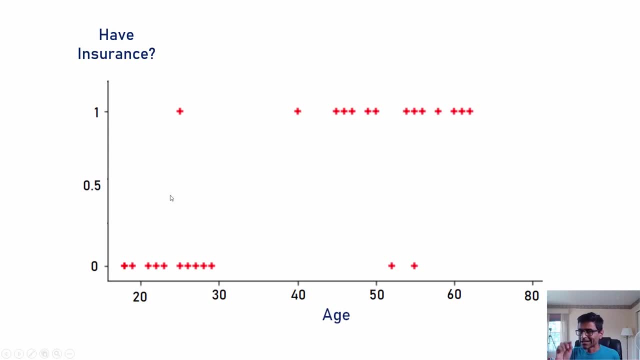 one means person have insurance. now again, going back to my machine learning tutorial playlist, using logistic regression tutorial playlist, i'm going to show you how to do this. using logistic regression tutorial playlist, i'm going to show you how to do this linear regression. you can draw a best fit line that goes through these data points, like this: 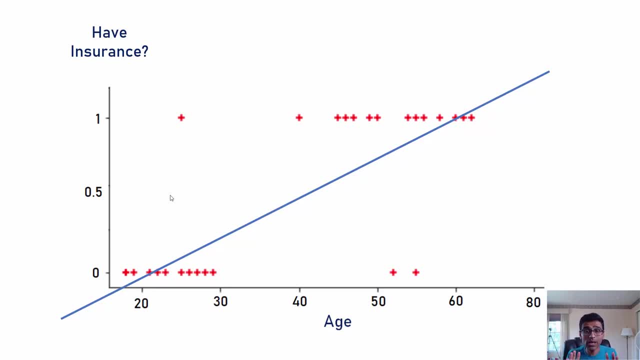 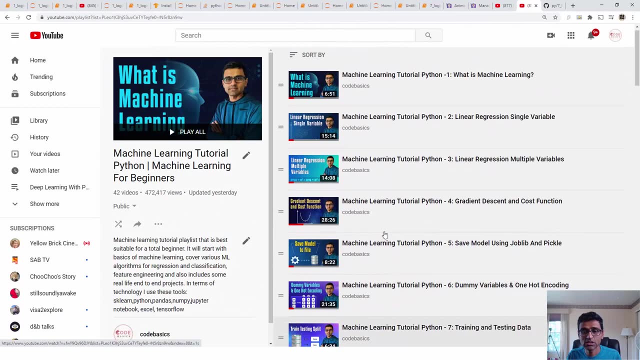 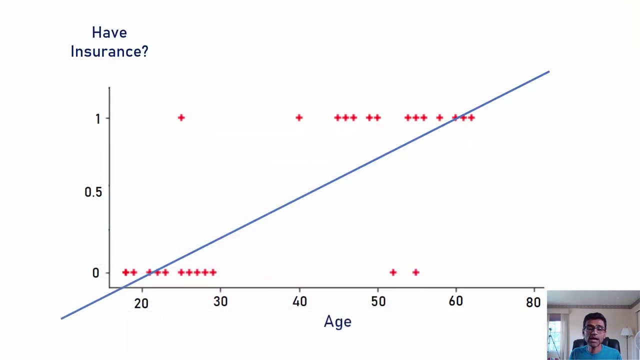 now you'll be like: how did i draw this line? well, there is this concept of linear regression, linear regression. if you don't know that concept, again, go to my tutorial playlist and follow these two tutorials, tutorial number two and three. they talk about linear regression, so, using that, you can. 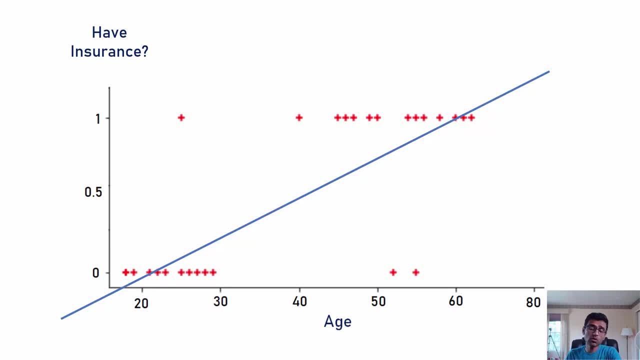 draw a best fit line. see, if you want to draw a single line that passes through all these data points, it's not possible, so you have to somehow come up with the best fit line. so this is that best fit line and after you draw that best fit line, you can do. 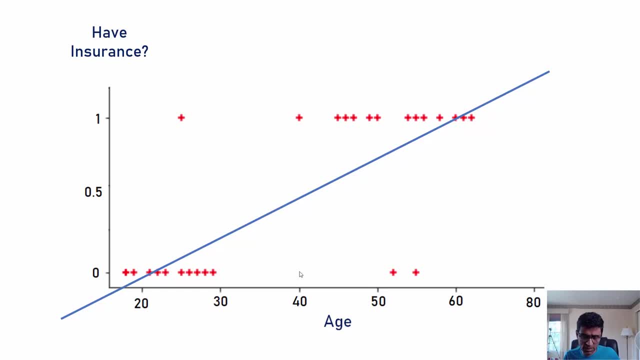 something like this. okay, so i have this line, which is my prediction function, and let's say i want to predict if an 85 year old dadima or grandmother want to buy an insurance or not. so here, where is 85? okay, let's say, i want to buy an insurance and i want to buy an insurance, and i want to buy an insurance. 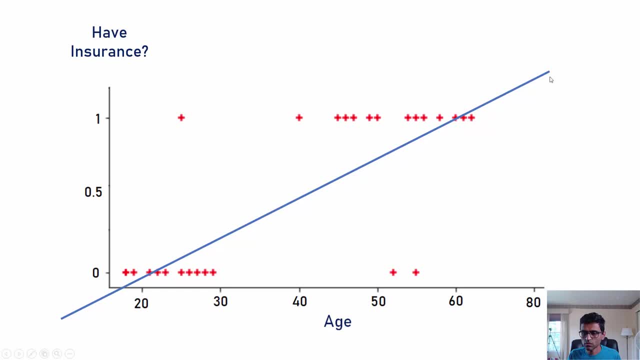 let's see on x axis: 85 is here. so if you look at this data point, it is more than one. so anything more than 0.5 person will buy the insurance. so you'll be like, yes person will buy the insurance, so you, anything which is 0.5 or up person will buy the insurance. less than that person will not. 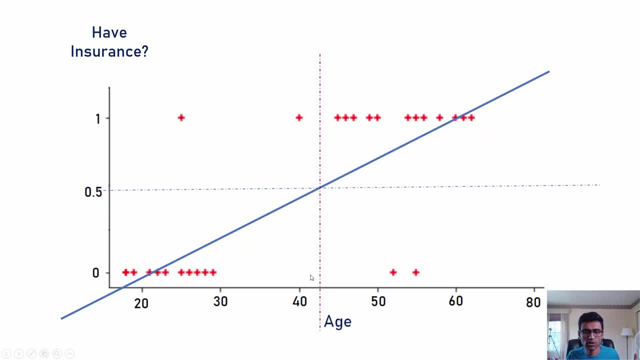 buy insurance. so then you get this red color boundary almost, so you can see on x axis: around 42 years of age a person starts buying insurance and then you get this red color boundary, almost the insurance. so linear regression, by the way, for this given problem, works perfectly fine. 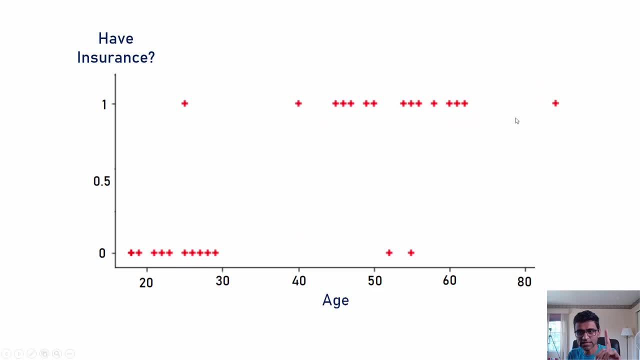 but there is one issue. let's say your data set has an outlier like this. let's say you have some very aged people in your data set who have had the insurance. now your best fit line when you are using linear regression will look something like this: and when you draw a boundary using 0.5, what? 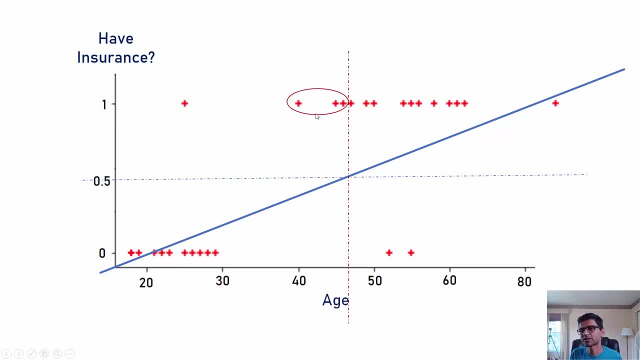 happens is you end up misclassifying certain data points. see all these data points. now your line will say: they do not need to have insurance because your age criteria has gone up. now it's like, okay, anyone who is 48 year old or more, that person buys the insurance. so you can see the 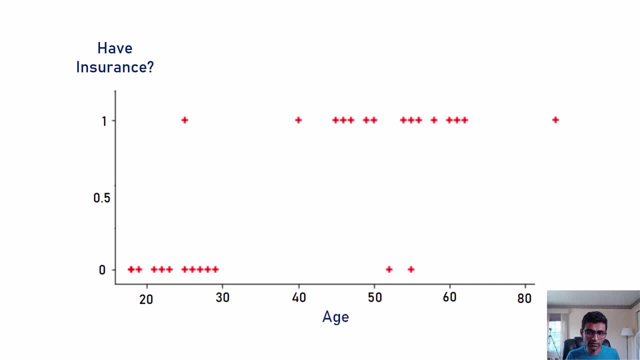 problem with linear regression here. what if i can draw a line like this? this line is much better. better because when now i draw my boundary, i will not be misclassifying those data points. of course, there will be some data points like this and these two guys. there will be some outliers, see machine. 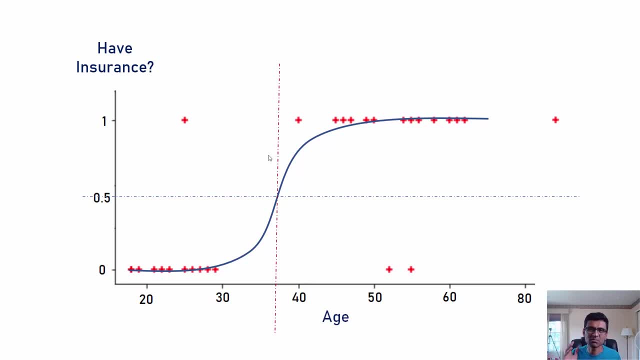 learning. all we are doing is some coming up with some best guess function. it might not be perfect and that's fine, but most of the data points this works okay, so this function is pretty useful. it looks like an s in alphabet. this is known as a sigmoid or logit function. if you have done some, 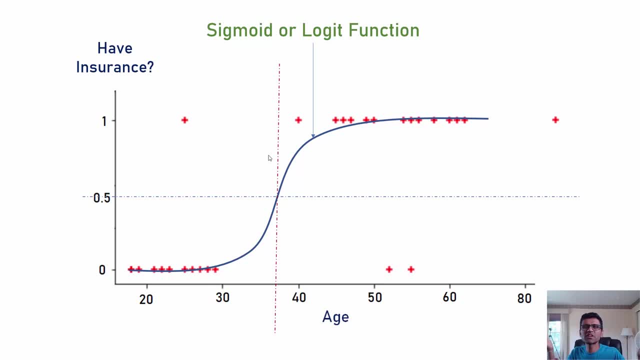 mathematics it is. it's just a name of the function. friends, do not worry too much about what is sigmoid logit like. whenever you hear mathematical terms i know you guys freak out, but don't worry, it's a very simple function as safe function, and the function equation is like this: 1 divided by 1. 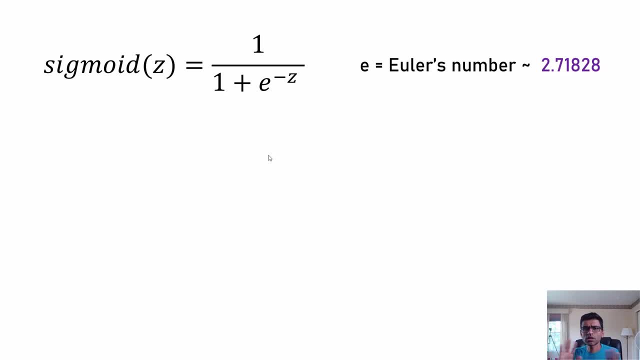 plus e, raised to minus 0, z is euler's number. what is euler's number? it's just some constant, like you know. how. about pi? how? pi is a constant number in the universe, same as euler's number 2.71. why is it 2.71? 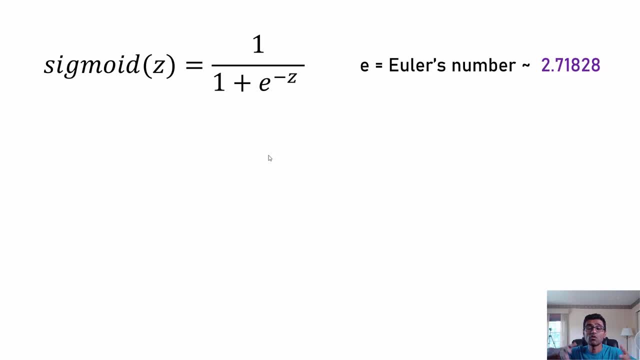 universe decided it to be that way. why do humans have two legs? or why do humans have two eyes? it's just some constant. universe has constants friends. euler's number is a constant. all this function is doing is converting an input value, z, into a range of 0 to 1. now look at this function. 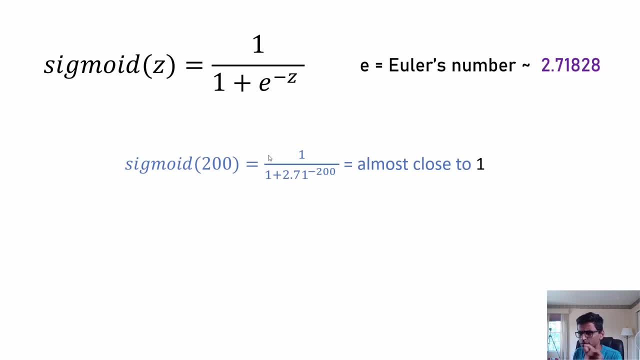 carefully. let's say you use this function for the value of 200. when you put 200 in the value of z see, this number becomes very, very small. so 1 divide by 1, plus very small, which is 1 divide by a number which is little greater than 1. 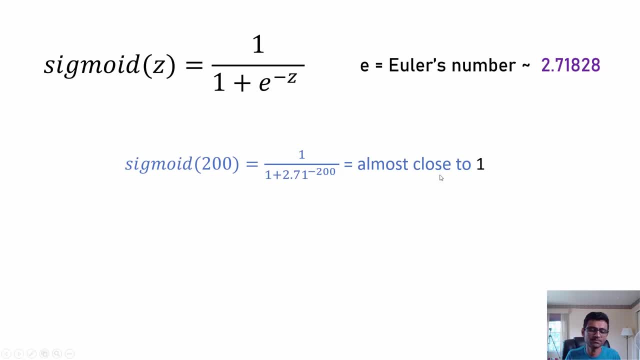 you will get a value almost close to 1. if you have a negative number, then this becomes really big and the number goes to 0. so all that this function is doing is take an input value and convert it between a 0 to 1. so if you have very like a bigger positive values, it will. 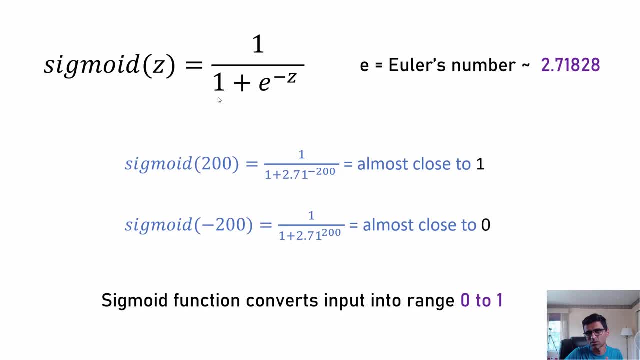 it will max them out to 1. it's like almost like a threshold: okay, value is goes beyond some point, it will just max it out to 1. value goes beyond certain point on a negative direction, it will max it out to 0. so any value you fade into this function, it is a simple function which will 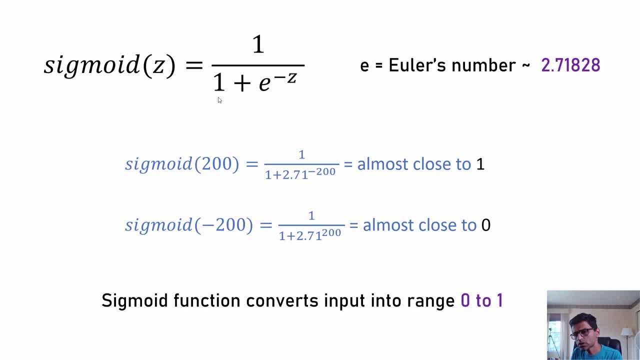 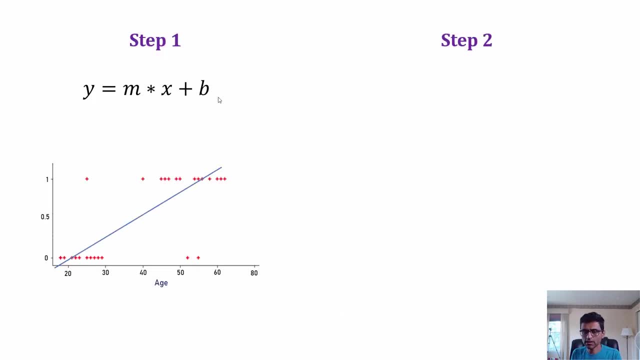 convert it to 0 and 1. and why do we do that? why do we need a sigmoid function like this? so basically we had, we have not two steps, so the in the first step we are still drawing a linear line using linear regression. okay, so y is equal to mx plus b, where x is actually an edge and b is some bias. so 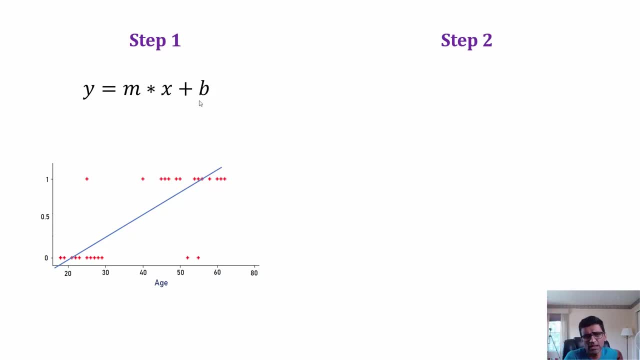 again. go through my linear regression tutorials. you will get an idea if you are still not sure about this mathematics. but the first step is you draw a linear line using linear regression. the line is y is equal to mx plus b, and the step two is applying a sigmoid function. 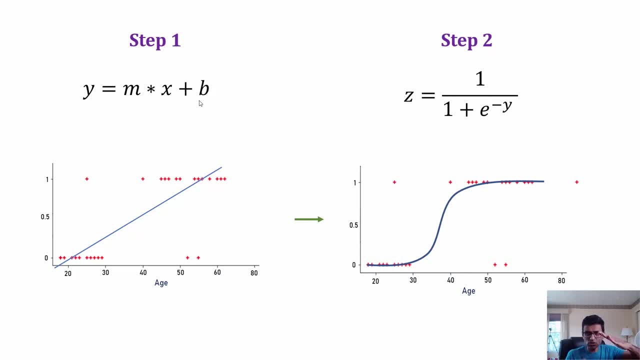 so sigmoid function is. you know, you have this line and you apply sigmoid function and it becomes like s, so sigmoid function is doing nothing. so it is taking the y from step 1, which is the output of step 1, and converting it into this nice curve, which is little better for our problem of. 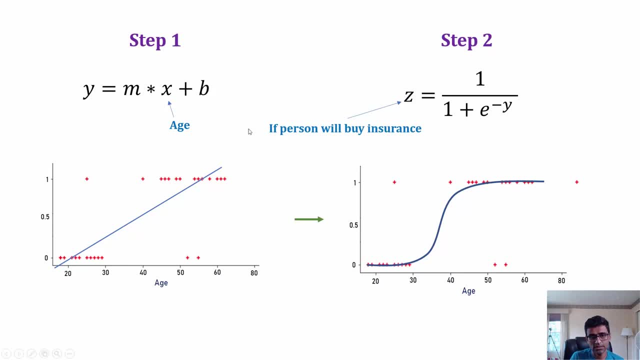 classification and if you look at X, it is an age, Z is nothing, but if person will buy the insurance. now, when you are working on a classification problem, all you want to know is 0 and 1. 0 means person will not buy insurance. 1. 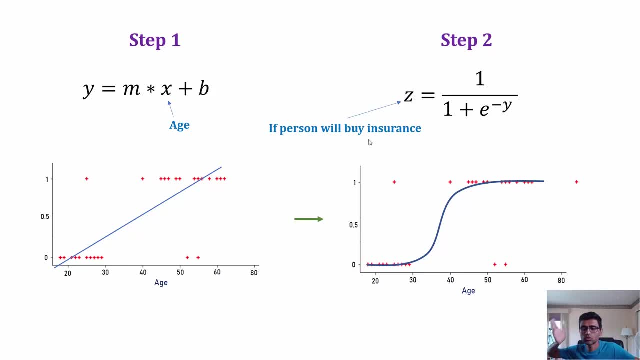 will put 1 means person will buy the insurance. so you are interested only in two outputs. remember from my machine learning tutorials: when you have a regression problem there is a continuous output, like housing price prediction, where you give bedrooms, square feet, etc. and you get a particular 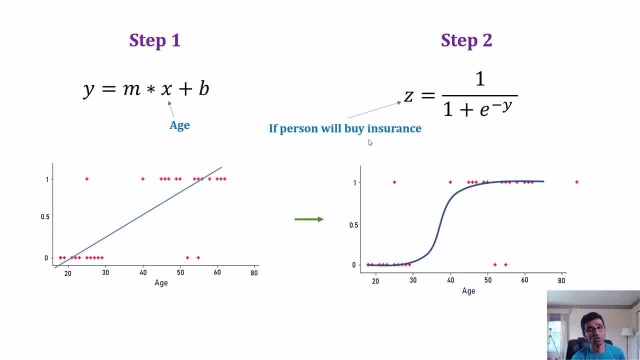 value like four hundred thousand dollars, five hundred thousand dollars. so there are values in regression, but in classification, like 0, 1, spam or not spam, categories basically. and sigmoid function is used exactly for that purpose, because it converts any value to 0 and 1 and what we can do is now: any value which is less than 0.5 we can. 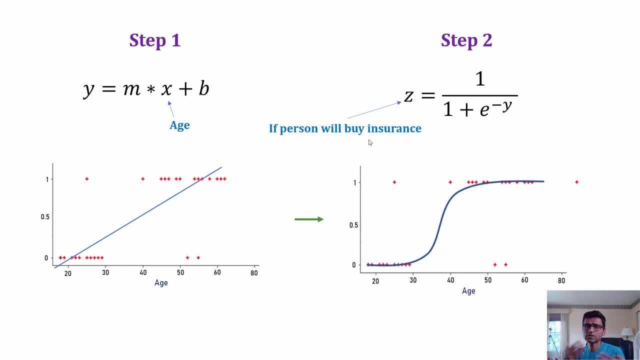 say it's 0, anything greater than 0.5, it's 1. so it helps you with a classification problem. now, when we look at our equation, when you solve this equation using linear regression, all you are doing is you are coming up with M and B. so let's say, in our case we came up with this M: M value is 0.042, B value is minus. 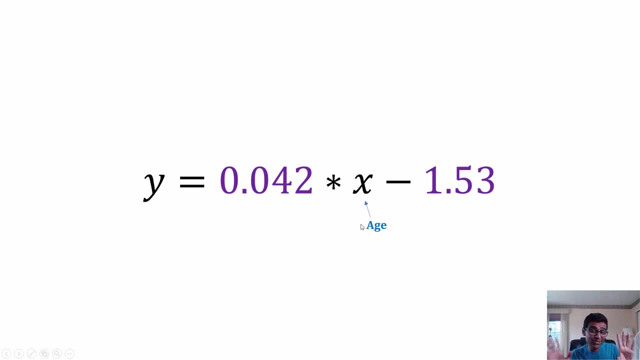 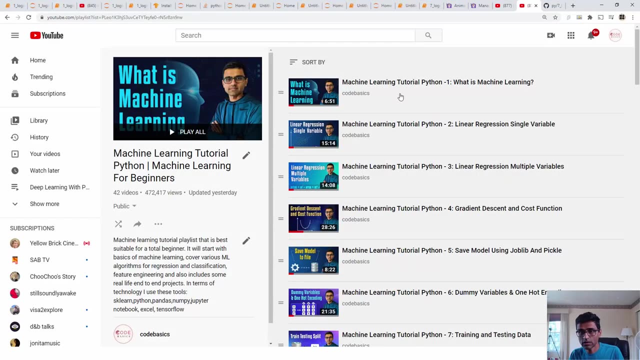 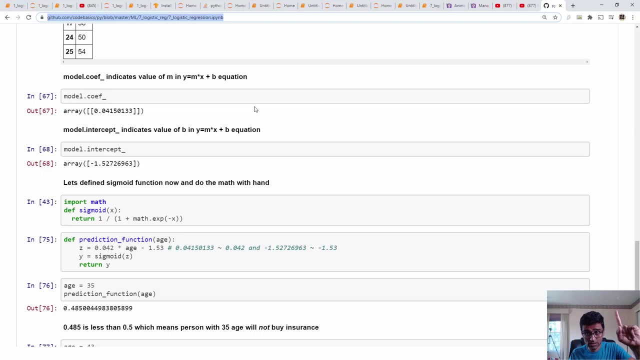 1.53. now, I did not randomly put these numbers, my friends. these are the real numbers for our insurance data set and, if you have a good memory, if you want to go to my linear logistic regression tutorial, which, again, I'm going to link in the 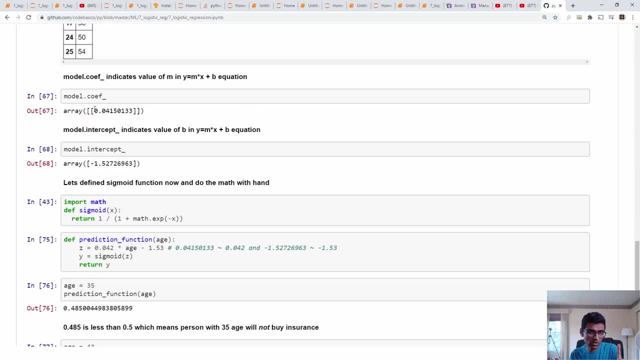 video description below you see these two constant. so the coefficient, which is M, is 0.0415, so you can round it to 0.042. intercept it is minus 1.527, so again round it to 1.53. so these are the numbers I. 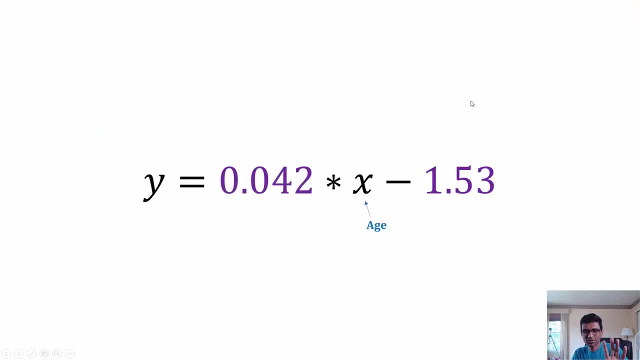 am putting on my ppt. I'm not randomly putting any number, okay. so now, thinking about step one and step two, we get this. so this is why that we calculate using M and B, and then the next step is Z, which is your sigmoid function. so now, once we have this two-step function, 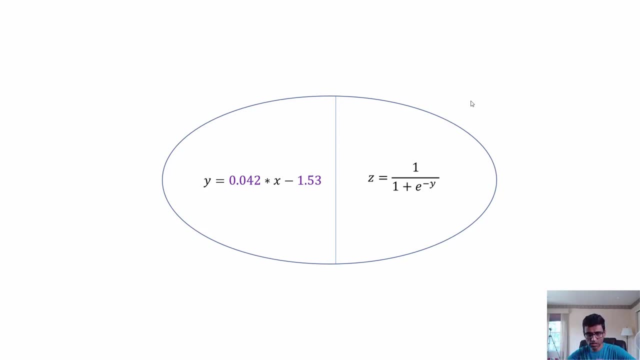 this is nothing but the logistic regression. okay, so we are doing logistic regression in this circle. so when you give, let's say, H 35 to this function, it will first calculate y and, by the way, you can put 35 in the value of x and you can have a calculator just compute the value and you will get 0.48. again, i'm not randomly. 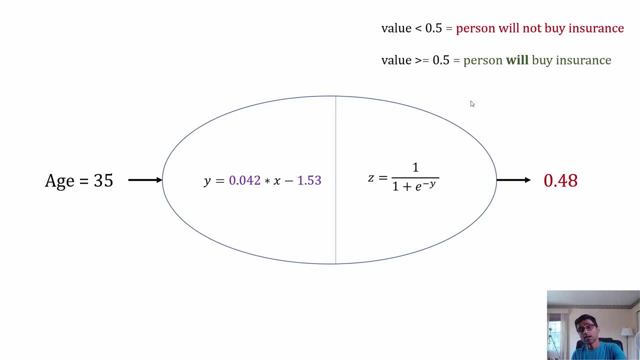 putting these numbers. these are the accurate numbers. and then step two is sigmoid function. so now, when you have 0.48, it is less than 0.5, which means person will not buy the insurance, hence the red color. i use red color with a purpose here. and when you have h40t 43, you get 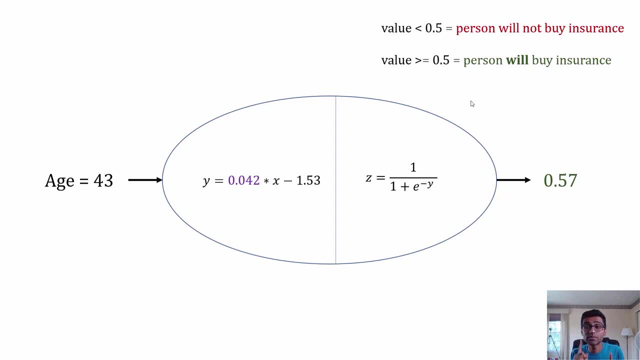 this value 0.57, which is more than 0.5, which means person will buy the insurance. yeah, you won a lottery. so now this already looks like a neuron. so this particular thing in the round is nothing but a neuron. neuron has this linear equation as a first part and an activation function as a second part, so 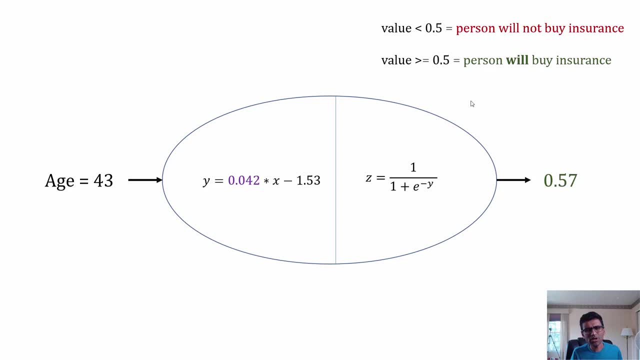 activation function is nothing but our sigmoid function. what does activation mean? you know you have those led lights at home. so when led light activates, it is on, when it deactivates, it is off, which means 0, 1, 0, 1, 0, 1. so sigmoid function is exactly doing that. you give any value, it converts. 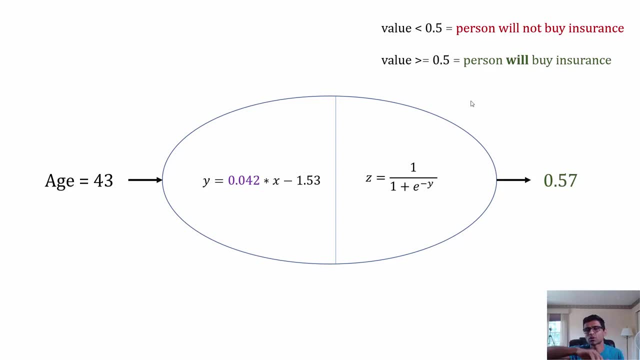 it to a value between 0 and 1, which means you can classify. okay, so this round here is nothing but a neuron. so logistic regression, you can think of it as a simple, like a single neuron. okay, now we used only one feature, so in the machine learning terminology the age is called a feature or an. 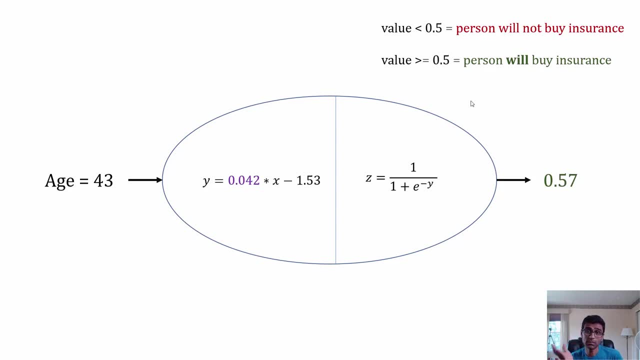 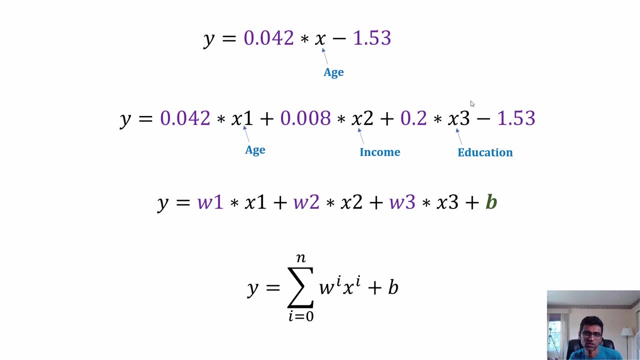 input parameter or an independent variable. the dependent variable is if person will buy insurance or not. now you can have multiple factors. actually you can have instead of age, you can have age, income and education. so you can have something like this, where in this particular equation let's say if i have income and education, because sometimes person, if person's income, 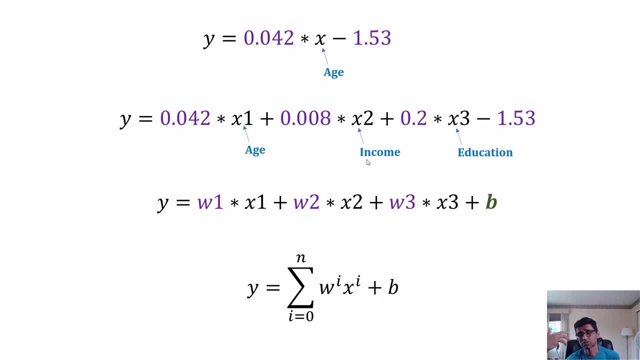 is high, then he will buy the insurance. okay. so person will buy the insurance or not might depend not only on age but on income and education. if a person is not educated at all and doesn't have health awareness, he or she might not buy insurance. so when you have 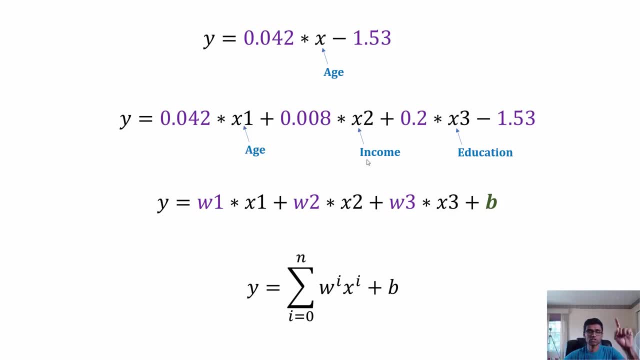 this kind of data set where you have three features, which is age, income, education, then you might come up with this kind of equation now, this time, by the way, 0.08 and 0.2. i just came up with this number out of thin air. i did not do any math here, just putting some numbers and generic way of. 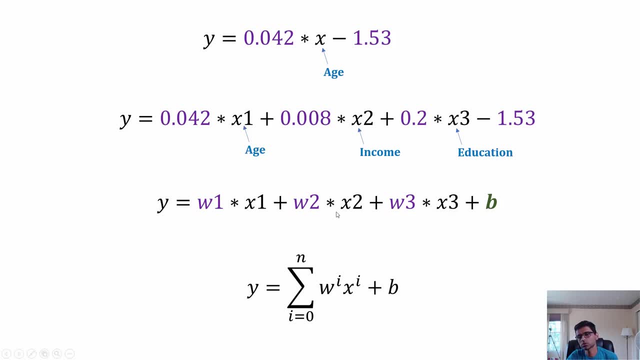 representing this equation is w1 into x1, w2 into x2, w3 into x3. so these numbers, the constant that you had, 0.042, 0.008, those are called weights, w1, w2, etc. x1, x2, x3 is nothing but the features. 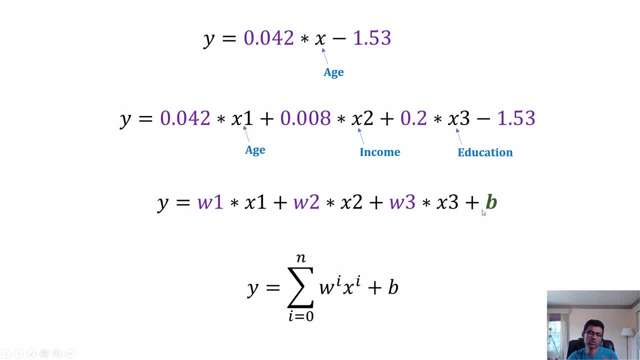 the features of your data set, and b is some constant number bias that you saw already in linear equation. in mathematics, generic way of representing this equation is this: so you are doing: a summation of i is equal to 0 to n, the i have n because i am showing three. 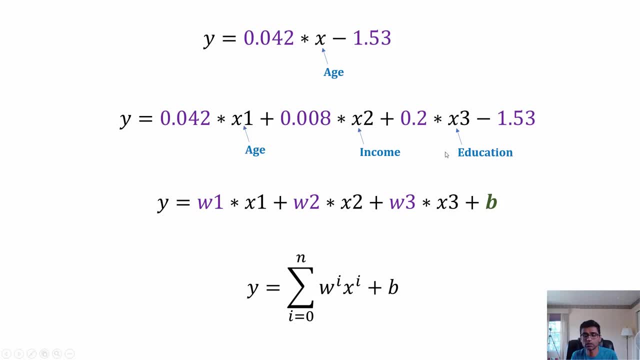 three features here. there could be five features, there could be 10, there could be 100 features. who knows generic way to represent this? is this: summation of 0 to n, wi into xi. so it is w1, x1, w2, x2, w3, x3 plus b, and that's when you get your y. 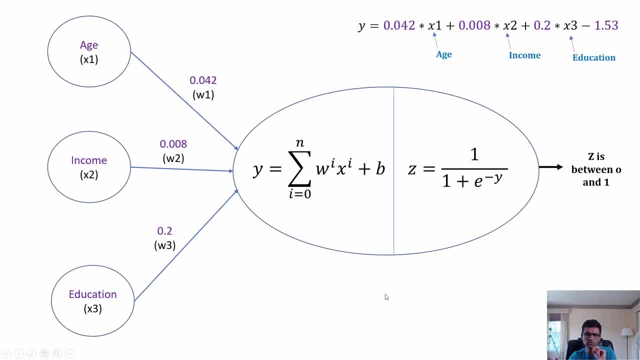 now, if you want to represent same equation in terms of neural network, you can present it like this: where you have this single neuron, which is your logistic function, you have the input parameters or the features, which is age, income and education, and the way you represent them is x1, x2, x3.